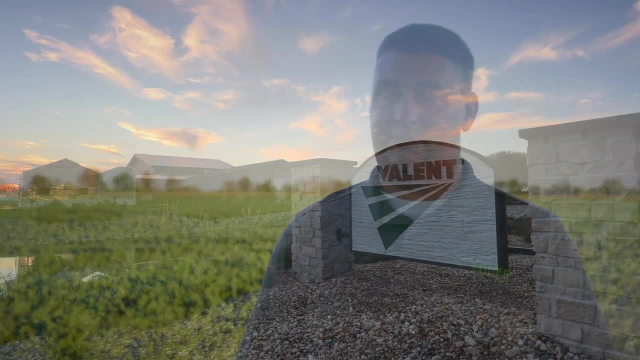 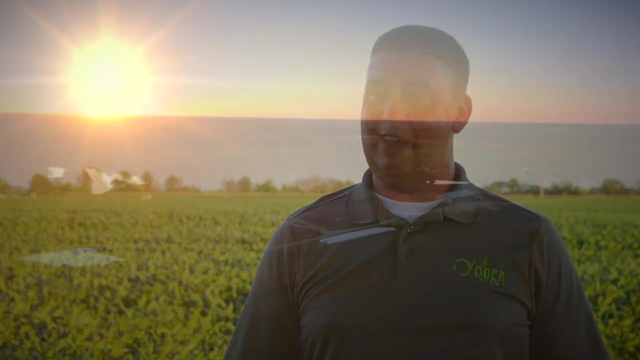 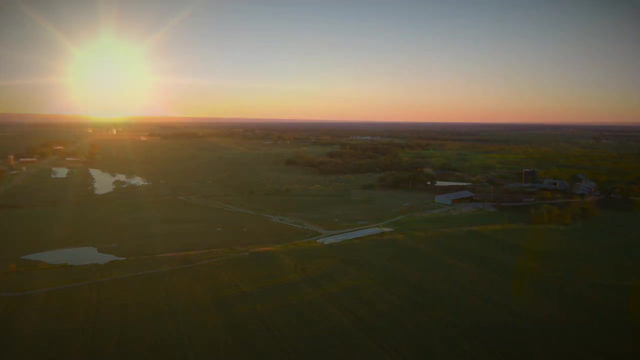 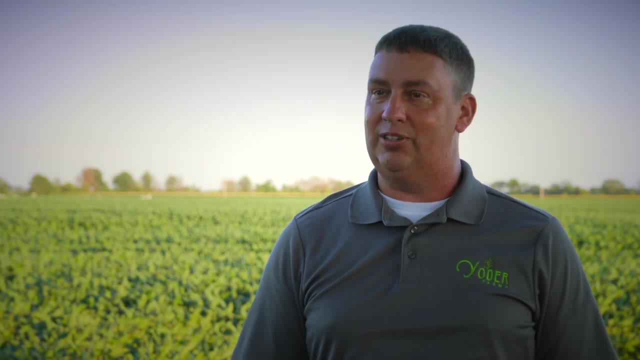 So they have the longevity into the future. From a young age my dad had always taught me the importance of conservation and protecting the soil and the resources that we have and trying to be as efficient and most productive that we can. And when I moved back, my dad was starting to implement some conservation practices. He'd been big on terraces and tile and those types of things but was just starting to dabble in the no-till just a little bit. So as I and my brother moved back, we made it a priority to try to implement a 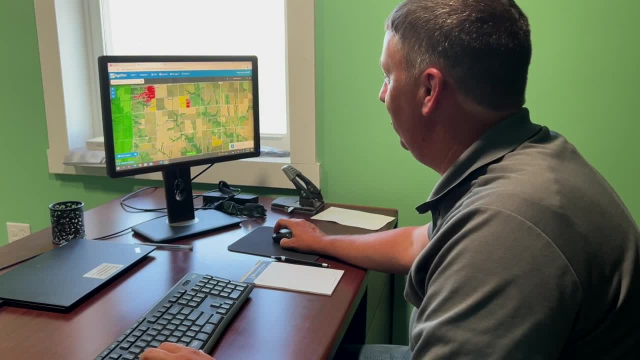 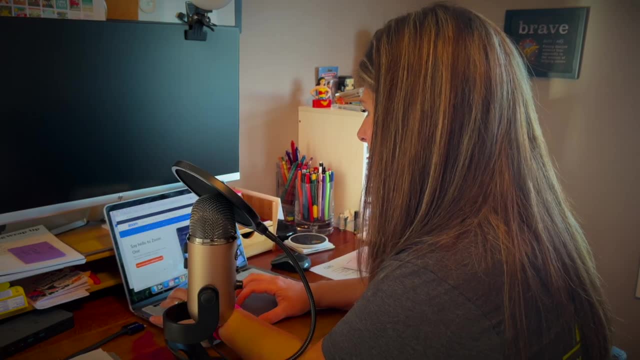 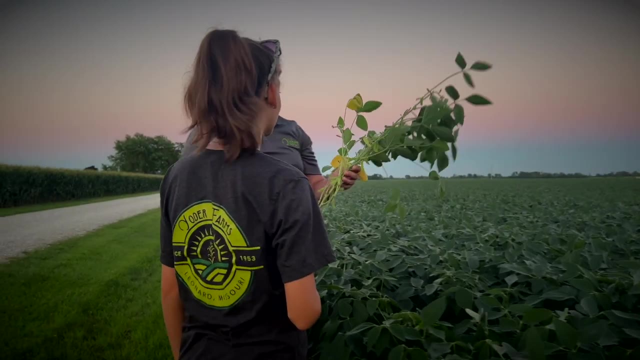 more no-till. We got involved with cover crops Through our interest in that. Addie and I got involved with the Soil Health Partnership several years ago, which has led us to be involved with some strip trials of cover crops, trying to compare what happens in the soil when you have those cover crops grown year in, year out versus areas where you don't grow those cover crops, and what's the differences between the two. 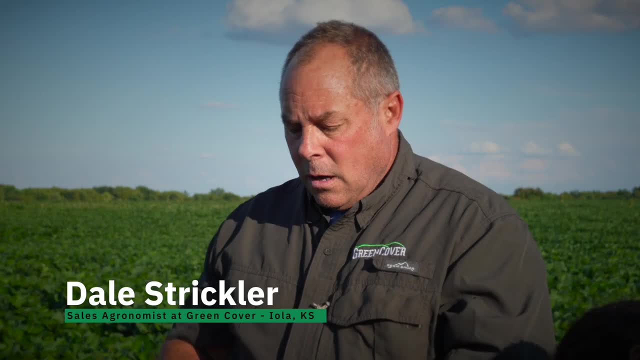 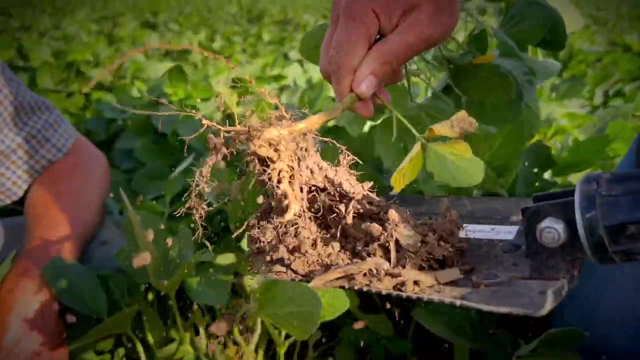 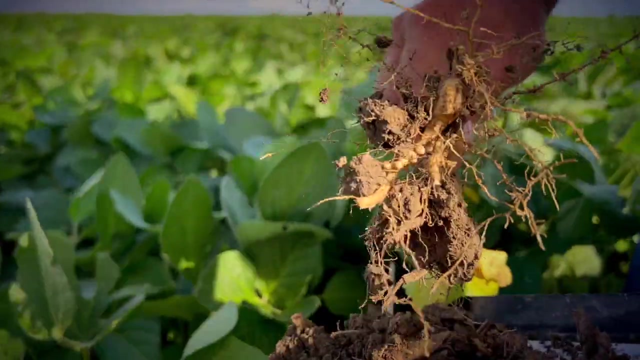 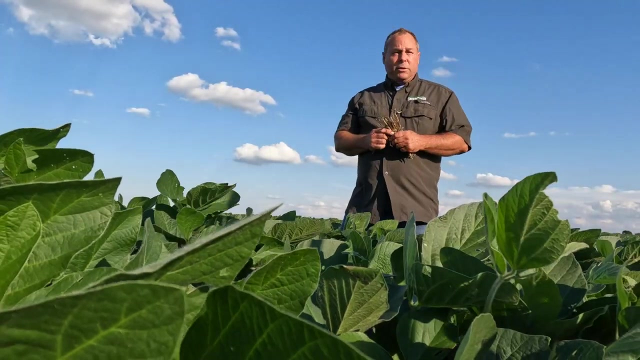 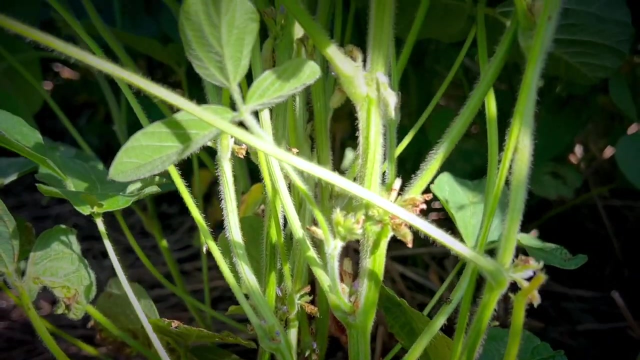 Two things really make the big difference on cover crops. One is the mulch that you create, and the second is the root exudates. The root exudates are really where you get your soil organic matter, and no matter what's wrong with your soil, you fix it with organic matter, And that comes from root exudates, And so you need to have a growing root in your soil at all times, And then you have the mulch. The mulch is what gives you your good moisture efficiency on your plant. 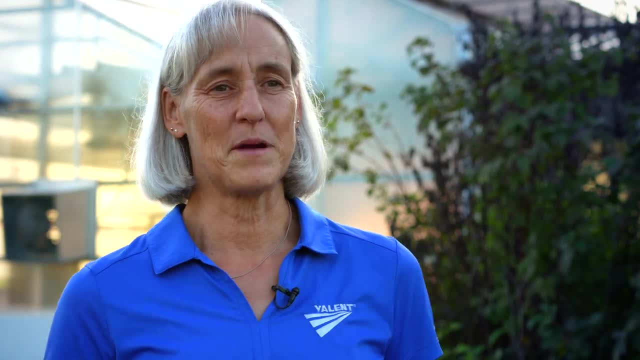 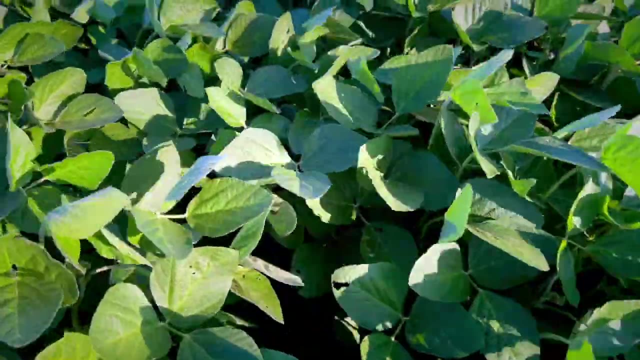 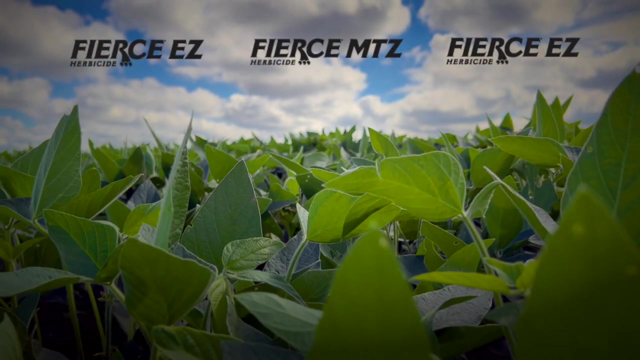 As we know, farming is stressful and Valen has a tremendous amount of products that can help that. It helps that farmer manage that stress, especially as they change practices to become more sustainable, to create more conservation practices on their farm And products like our Fierce family products, putting those on at the right rate at the 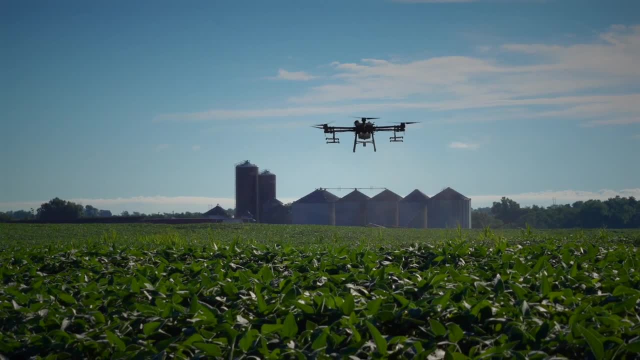 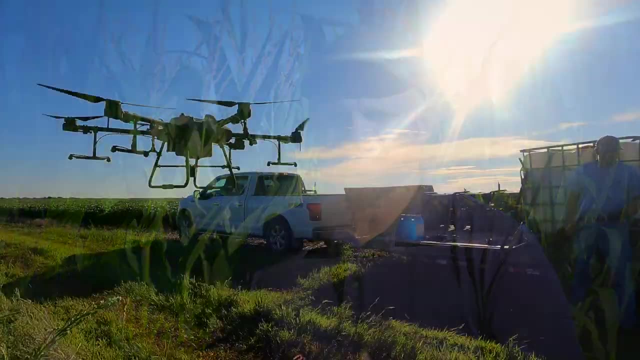 right time can really help that farmer do a better job as they're raising their crop. I think the equipment and the technology are what actually enables us to do the operation that we have today. You know covers are not new. People have used cover crops for many years. 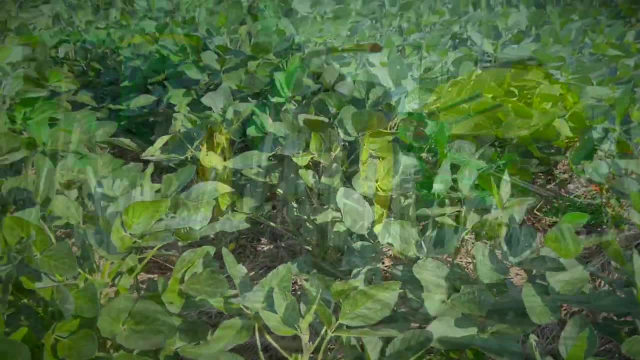 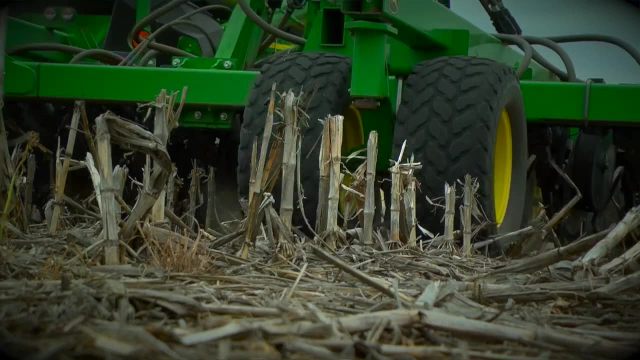 in the past, but they haven't always had some of the equipment. the no-till planters set up the way that we do today. All the nutrients that we can put on with a planter today allow us to handle that challenging situation.